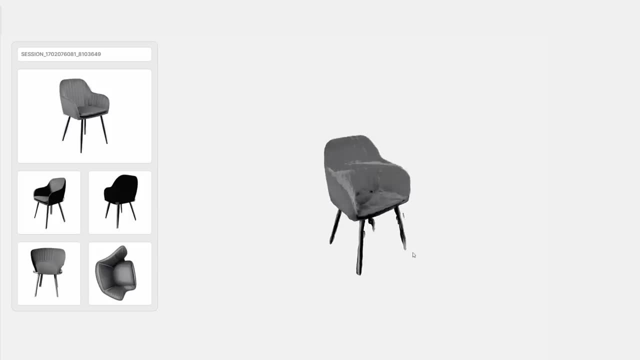 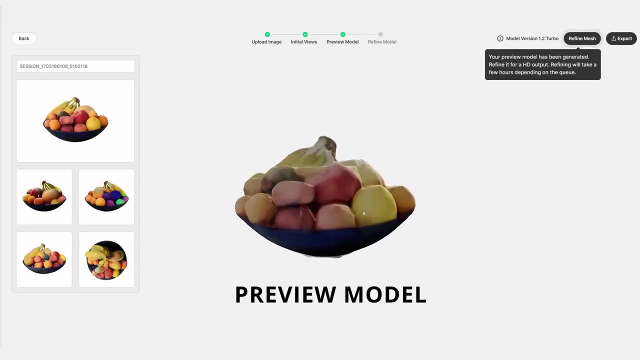 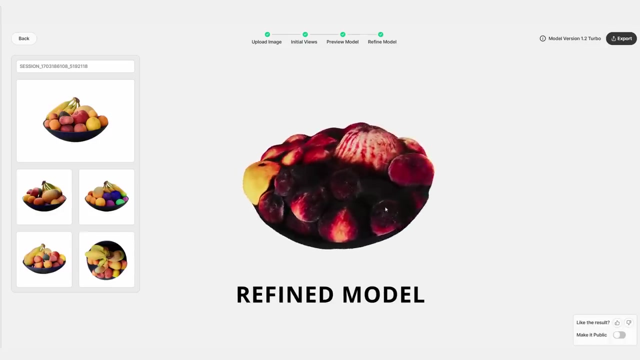 plain background so that your object can be easily identified by the AI. If you choose an image with a lot of different items, you may get less satisfying results, but to be honest, it's not that bad. To be honest, it is still amazing how even the complicated pictures can be analyzed with. 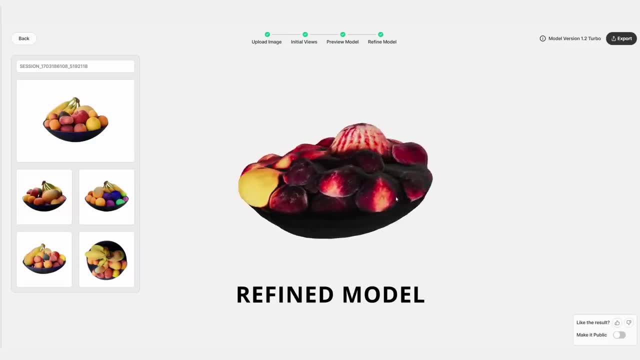 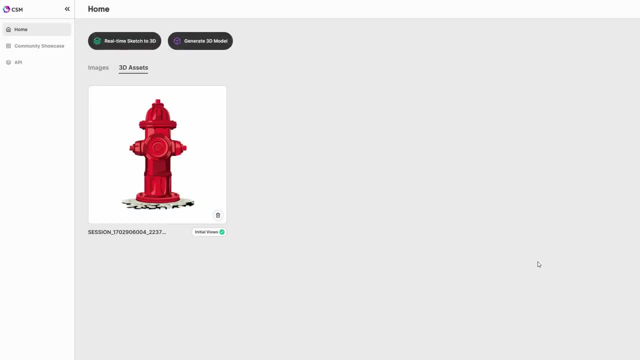 such a precision. I'm actually scared how fast this is developing. Once you upload your image, it will be added to 3D Assets in a form of a new project. Select it and enjoy the magic of the times you're living in. 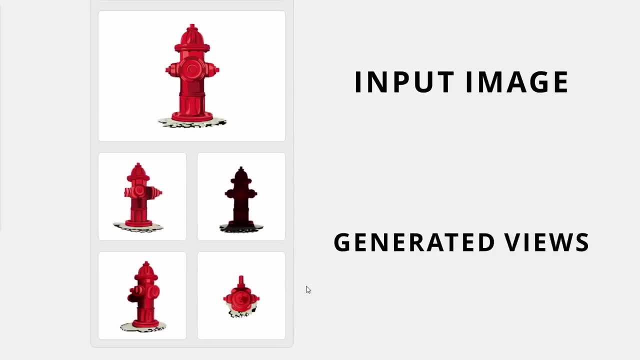 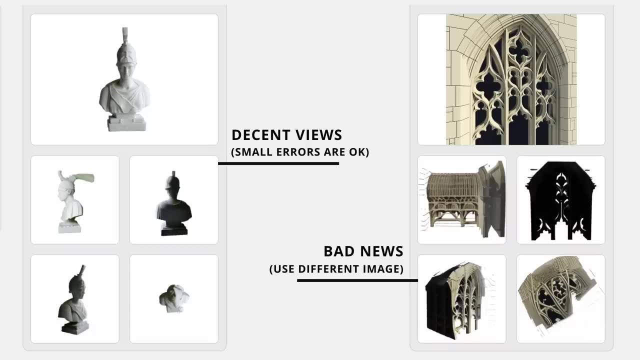 CSM has analyzed the object on the photo and created the estimated top side and back view. This is the moment for you to start working on your project. You can click on the top view to decide if the views are looking mostly accurate and if you want to proceed with this image. 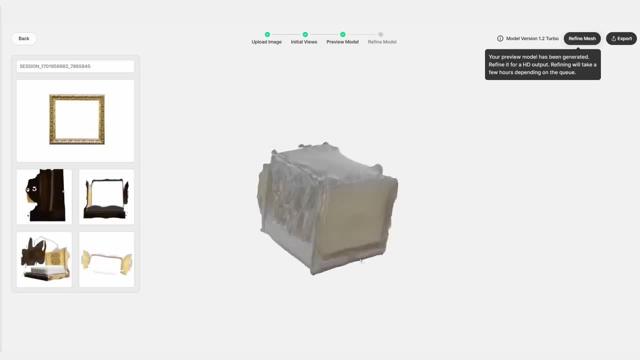 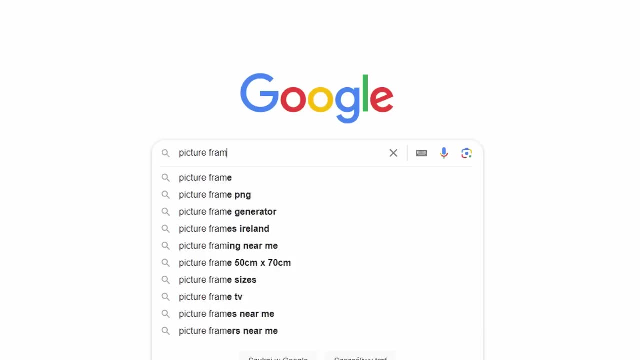 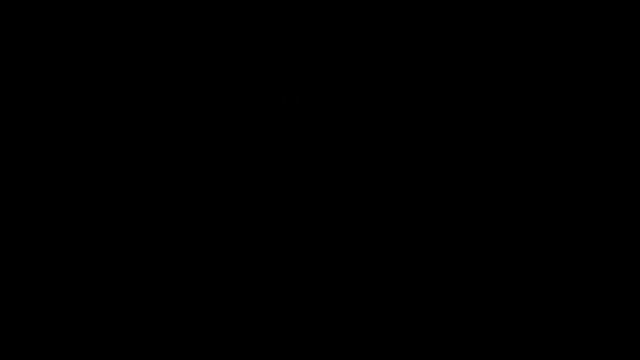 If, for some reason, the views are too distorted, that means the AI had a hard time with analyzing your image and you should probably try with some other photo. It doesn't necessarily mean the object you picked is doomed. You can try googling the same item with different background or perspective. 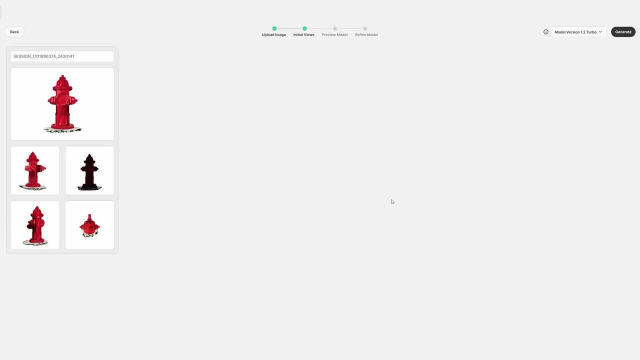 It may help quite a lot. However, if initial views are looking more or less okay, go ahead and click Jogging. You can also click Generate in the right upper corner. The simplified model is now being created, as the yellow dot informs us. 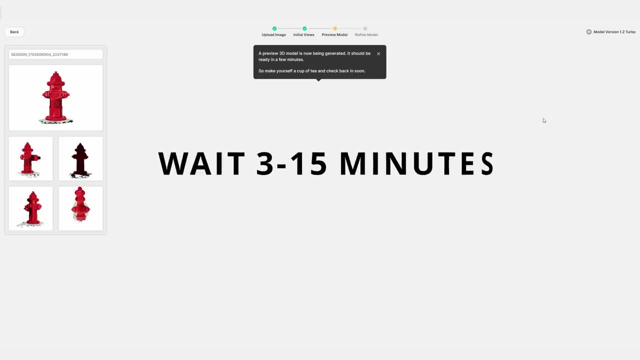 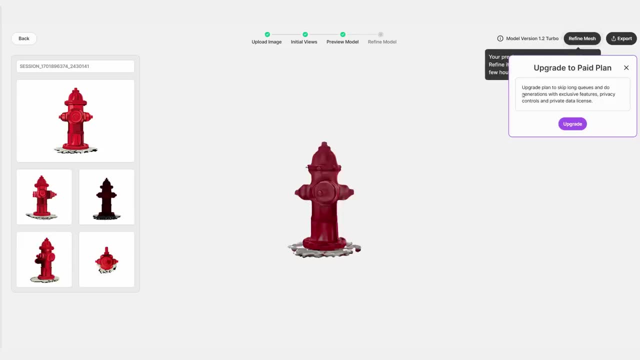 Depending on how many people are using this feature right now, this process should take anything between 3 to 15 minutes. When the work is done, you will get access to your 3D model. Use left mouse button to rotate it around, scroll to zoom and right mouse button to move. 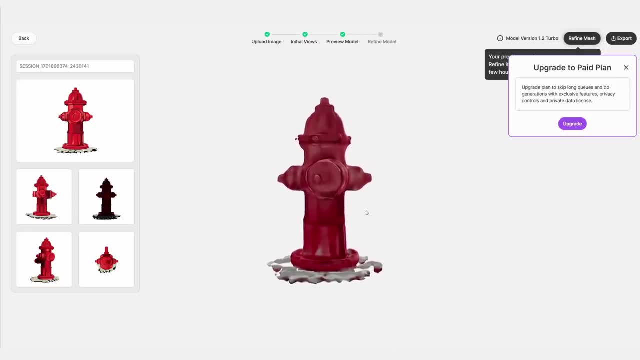 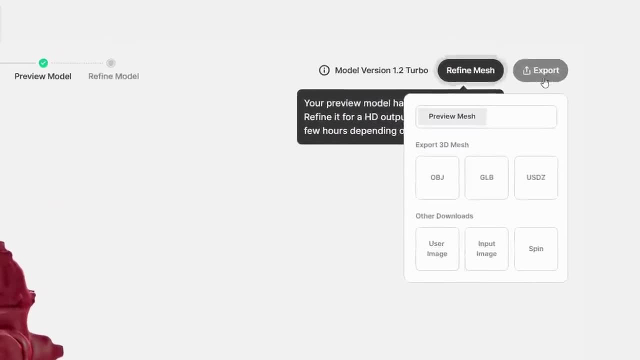 it. Keep in mind, this is just a preview. I'm not going to show you how to do it. This is just a preview model and you can make it even better. You can either download the model right now if you're happy with its quality, or go a step. 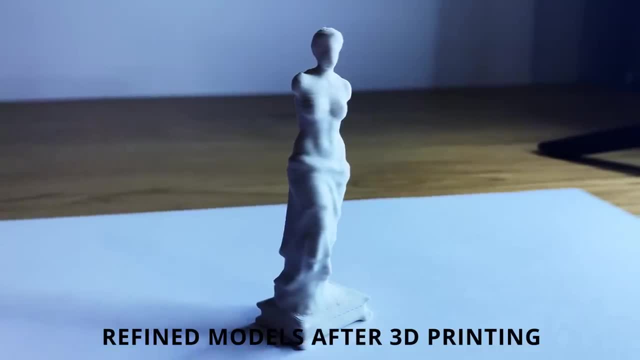 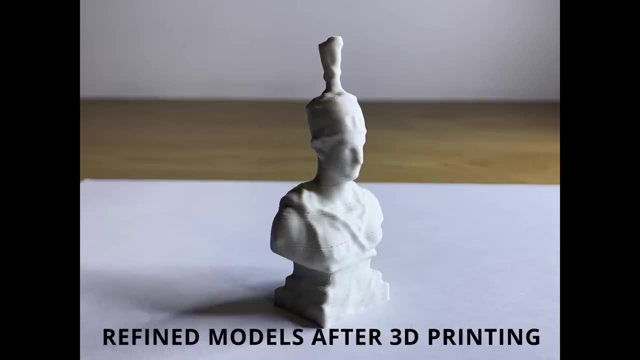 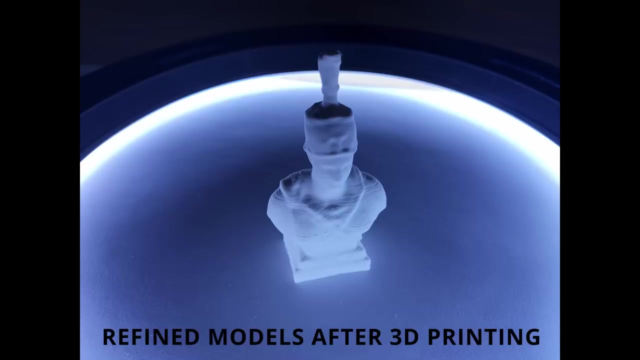 further and refine your project. It is going to improve your model even more, but it's going to take few hours to do that. The good news is you don't need to have your computer on during this process. I usually just leave it refining for the night and when I log in the next day, all the models 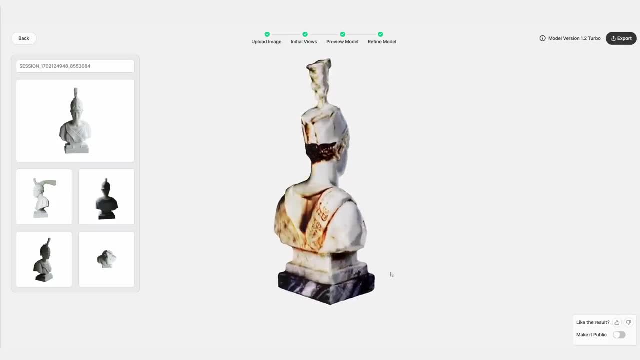 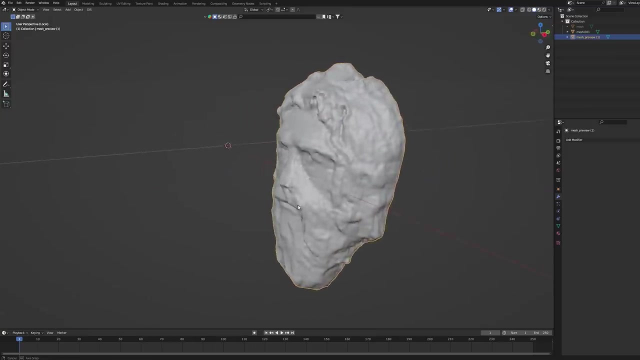 are complete. The quality is just amazing. It's hard to believe you can get such results for free. If you're wondering how significant is the difference between preview model and a refined one, here's a brief comparison. This is a preview model of Poseidon's antique sculpture. 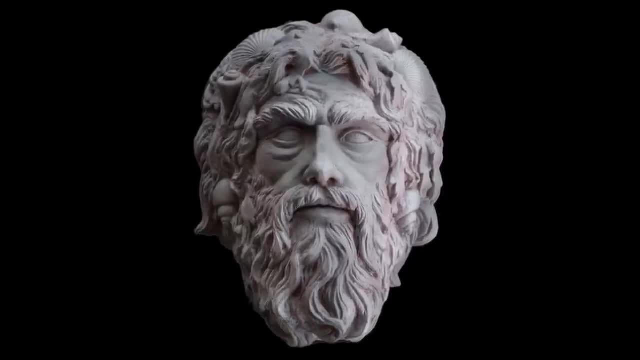 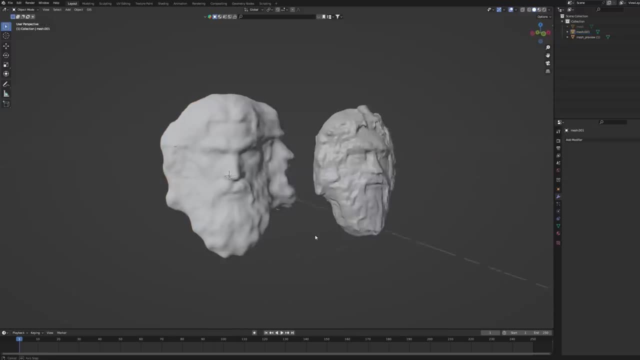 It's fully generated with the image I've found online And this is refined model. I've imported both objects into Blender so I can make some required adjustments before 3D printing them. And don't worry, I will teach you all of this process in a minute. 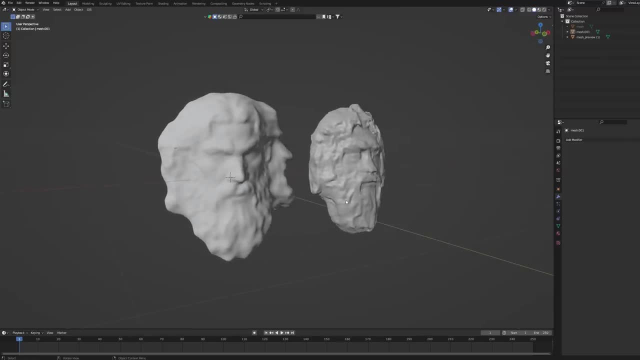 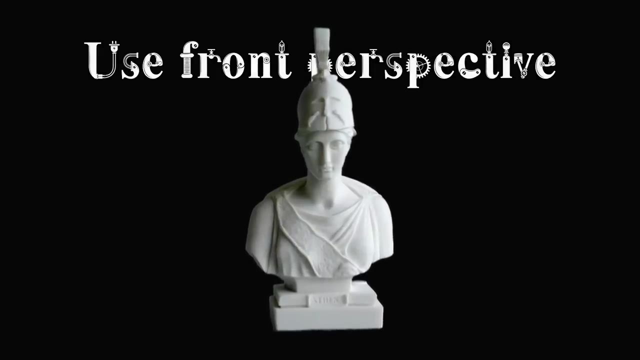 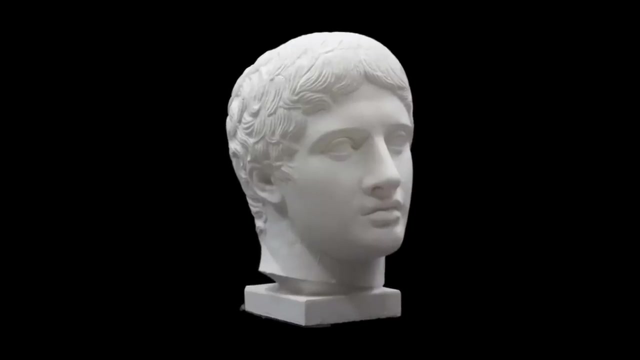 But first let me share a few tips on generating your own models From what I've learned after many, many tries. you should always try to find an image with your object facing the camera. Whenever I have uploaded, image with some tilted perspective, like characters turning towards. 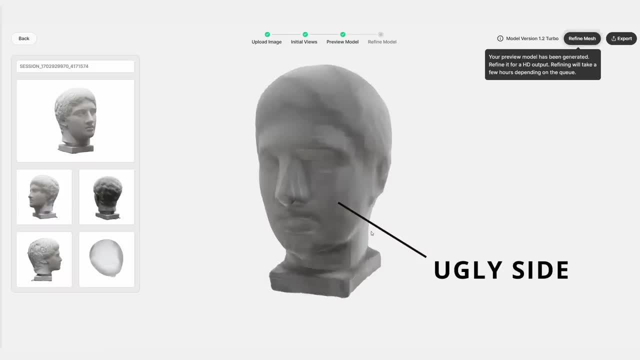 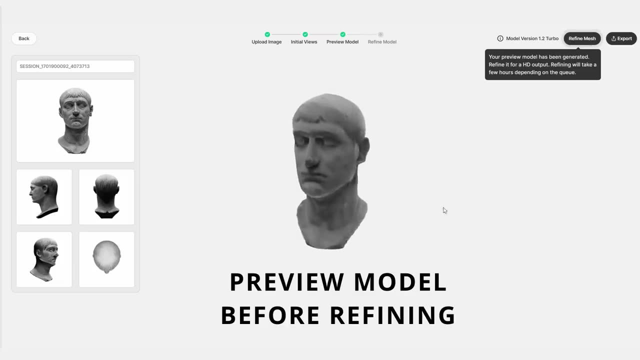 the viewer from the side. the AI had a really hard time with understanding how the back of the model should look like. If you have any questions, feel free to ask in the comments. If you stick to the front view images, you will get more satisfying results. 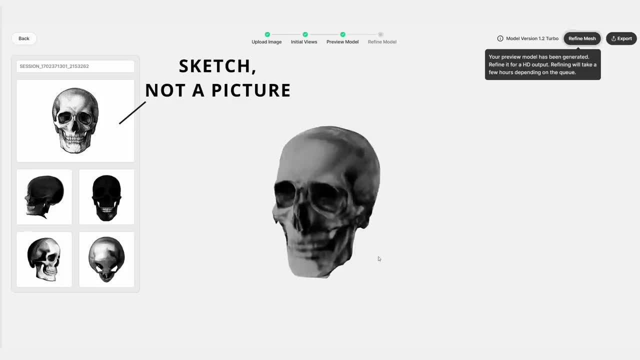 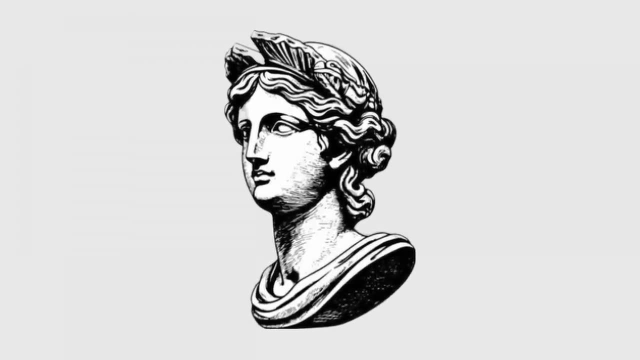 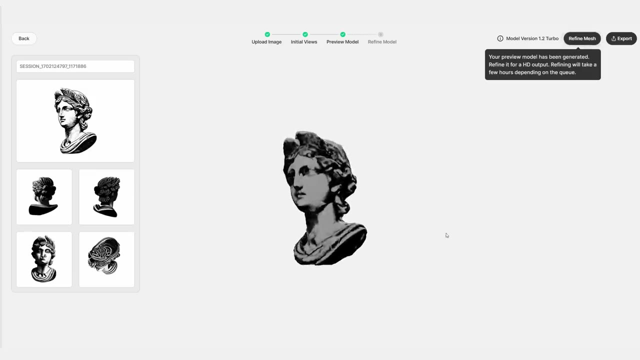 For the second tip, you may be surprised that CSM also deals pretty well with drawings and sketches. Even with shadows provided by nothing but a pencil on a paper, AI does pretty good job with understanding how the geometry should work in a 3D space. 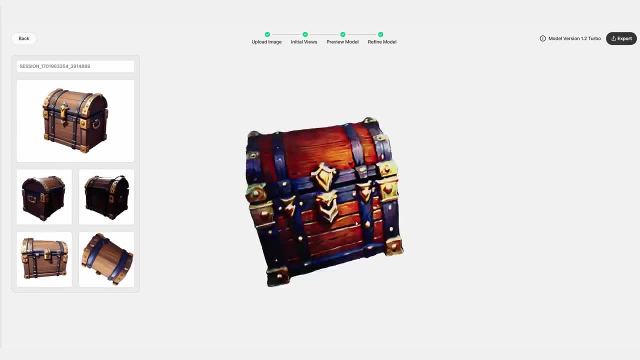 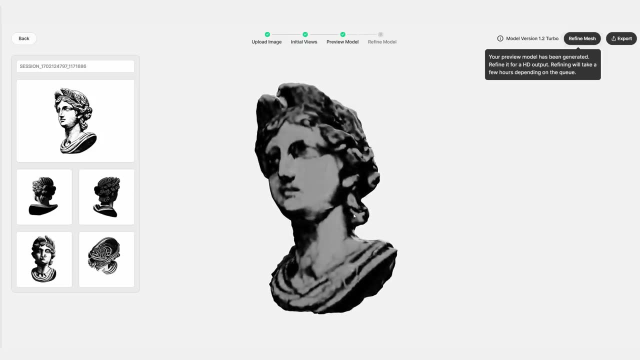 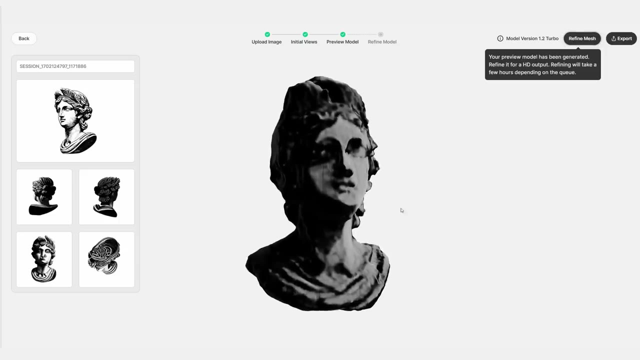 Your image doesn't need to be a realistic picture. It could be basically anything, So go and have some fun with that. By the way, this is also a great example to a previous tip. This character is not in a front perspective, so the geometry is distorted. 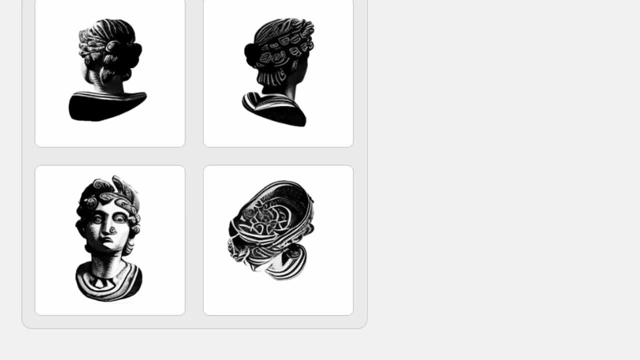 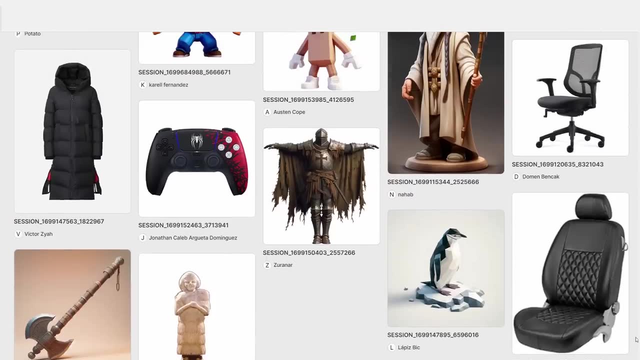 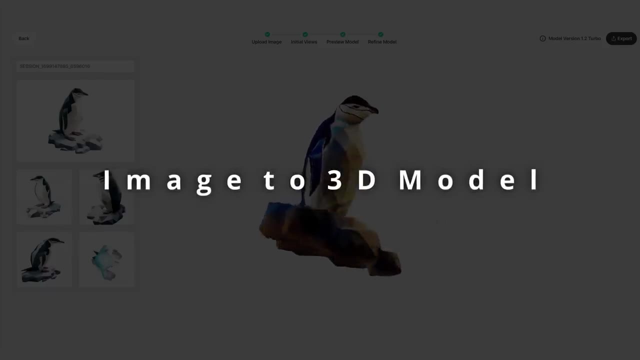 So to keep a clean outcome and save yourself from unexpected nightmares, just use a front view images. Third tip will revolve around choosing your object. You need to understand the limits of image-to-3D-model technique in order to utilize the most of it. 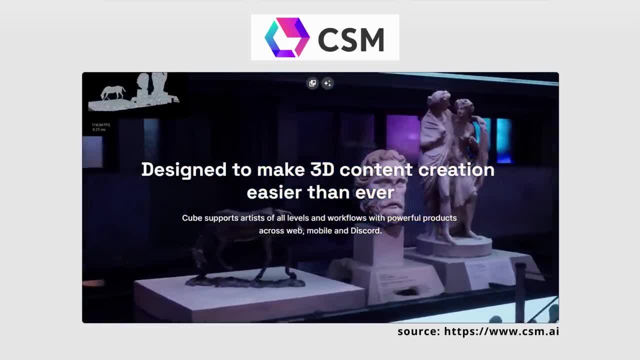 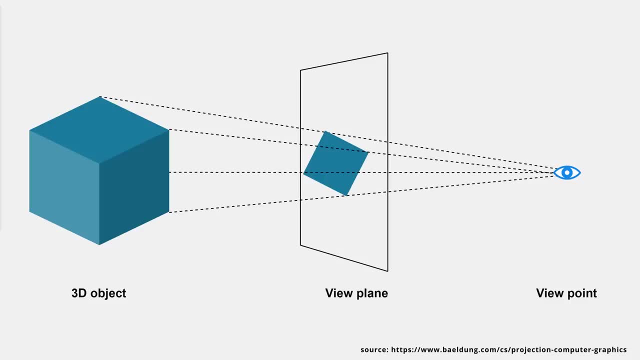 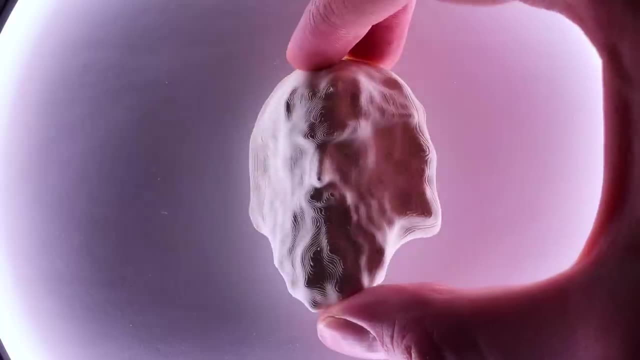 Tools like CSM can provide you with great looking models and really advanced geometry. however, this technology has its downsides. Basing on a picture which is a two-dimensional source, the AI can only estimate the 3D version to a certain point. 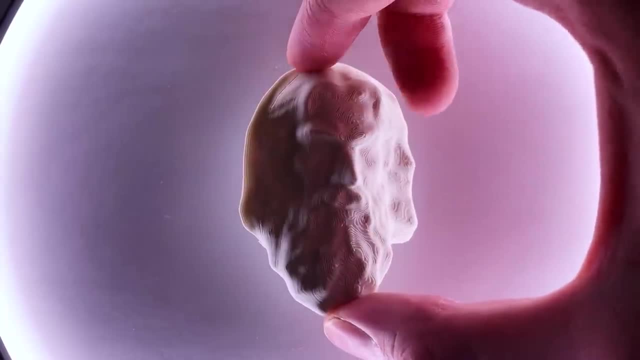 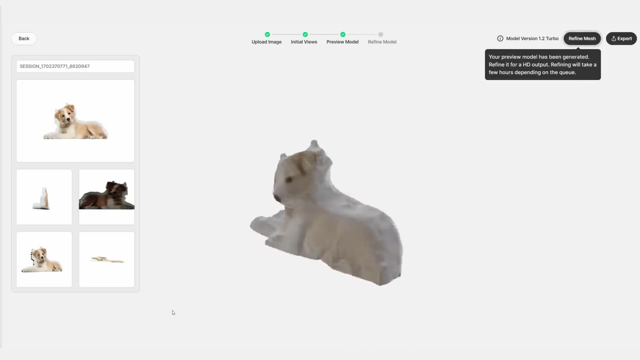 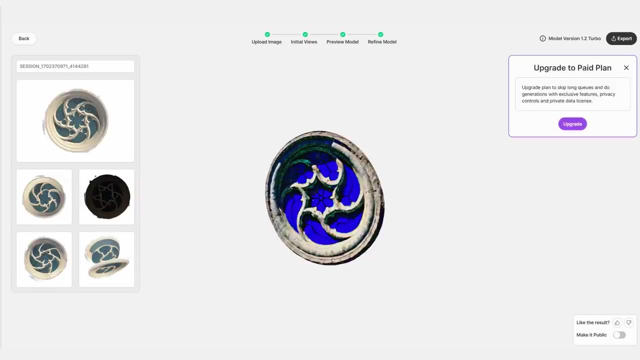 Therefore, when choosing the object you want to create, I would suggest going for rather flat items. The more information is missing on the picture, the more far-fetched the 3D model will be. For example, when I used these facial sculptures, architecture details or even whole statues, 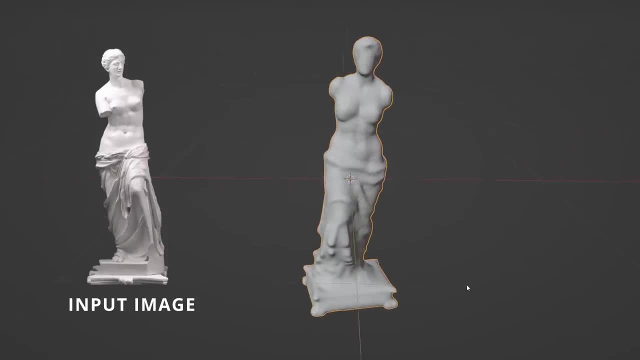 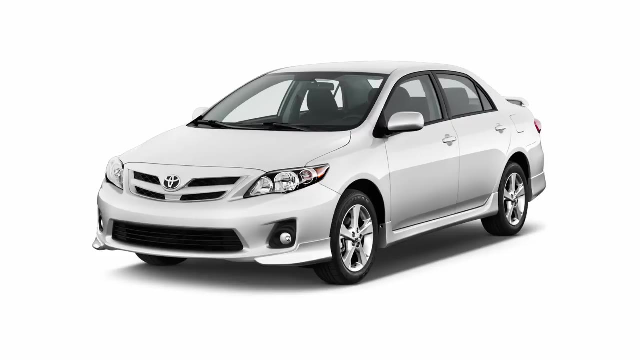 the results were awesome because most of the information was already in the image. However, when I used a front picture of a car which, as we know, has a lot of elements on its sides and back, the AI had too little information about that. 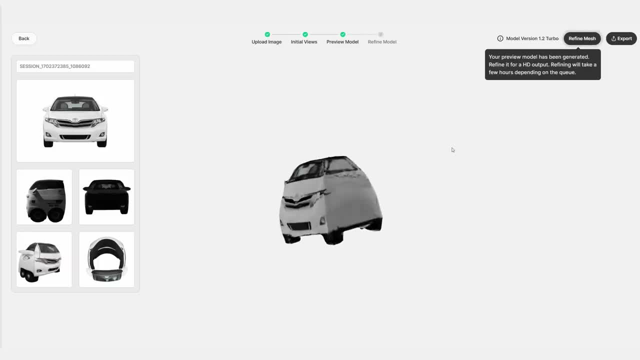 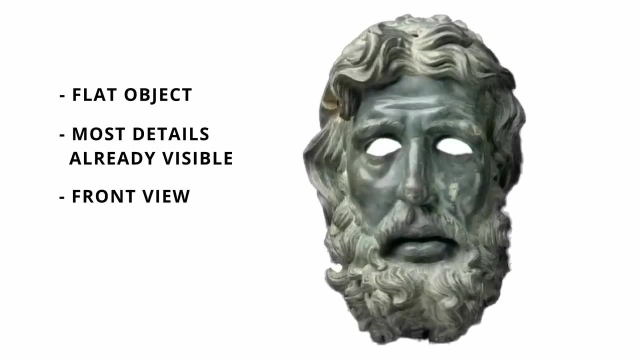 The whole object and could only produce this monstrosity. So as long as you stick to objects that can be easily described with just one photo, where most of the crucial information is already visible, you will have a great time with this tool. 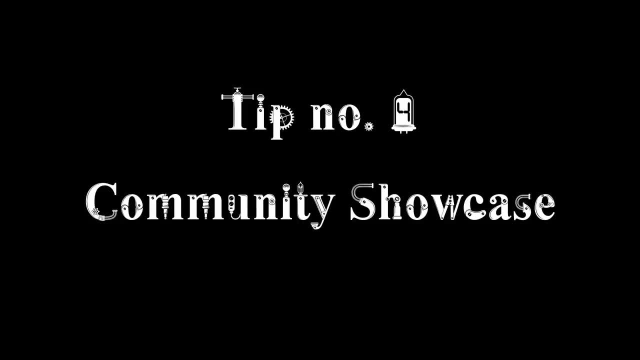 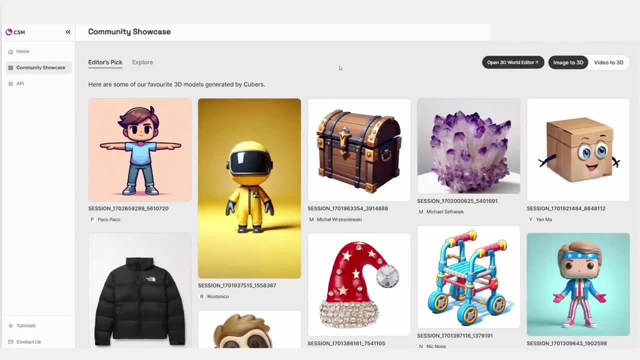 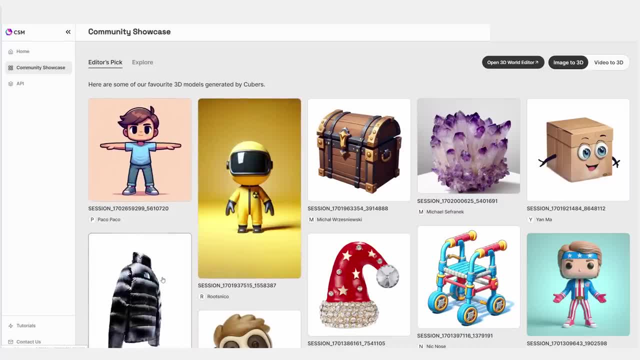 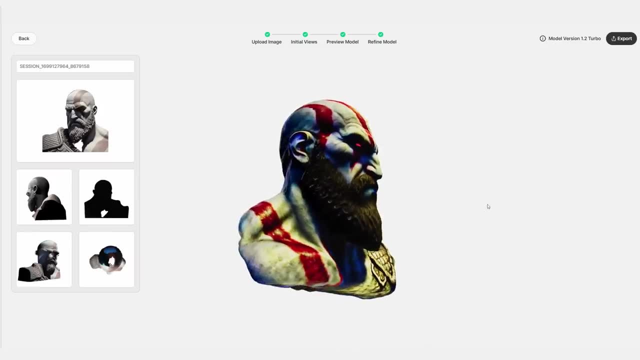 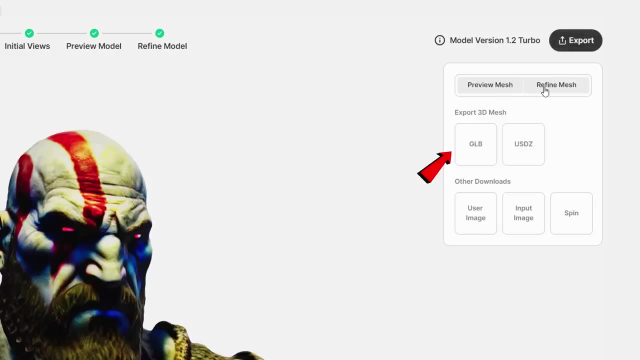 Not only is it a great source of inspiration, you can actually download any model you find here and use it however you wish to, Feeling like 3D printing Kratos bust from God of War Export. choose refined model, select file extension and there you have it. 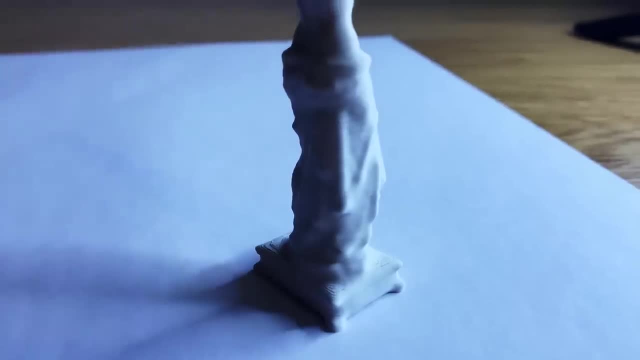 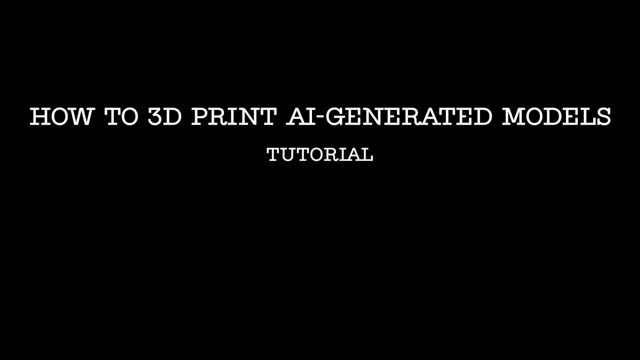 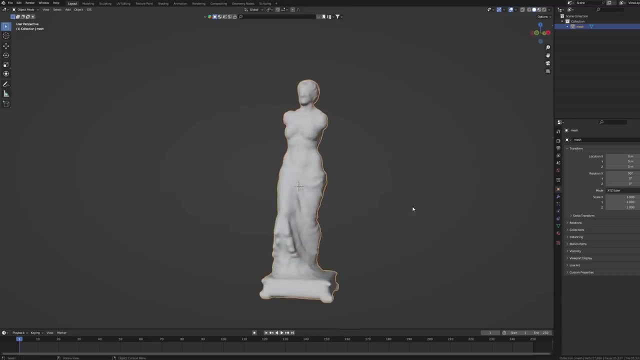 But how to prepare a 3D object like this one so it can be printed easily without any issues. Well, I'm glad you asked, because now I will show you my most efficient routine of 3D printing AI generated models. This part will cover the basics you should be familiar with in order to turn your models. 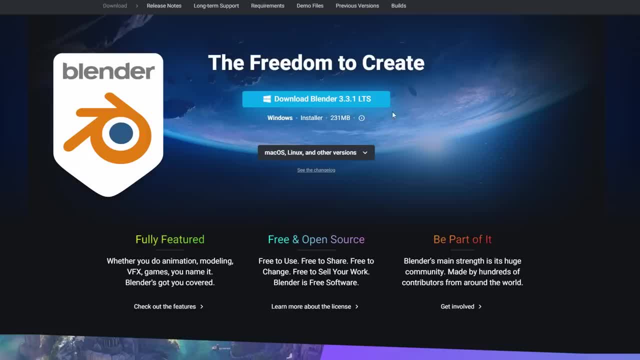 into clean and pretty 3D prints. We will use Blender, which is a free software you can download from the link in the description. Do not worry if it's your first encounter with this program. I will guide you step by step, and the whole process should only take a few minutes. 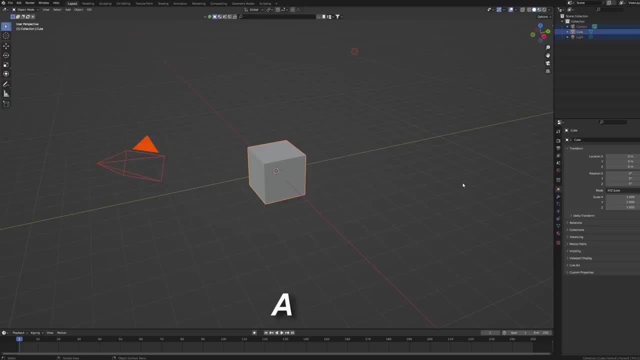 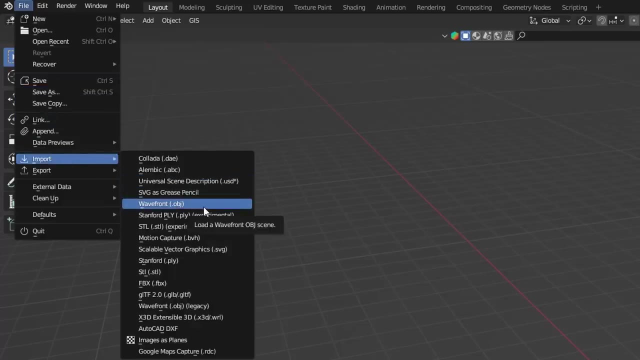 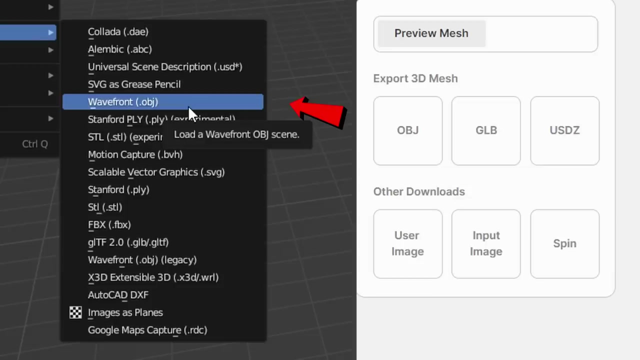 Once you open Blender, select the default objects with A And delete them. Go to File Import and choose the file extension you used to download the models from CSM AI. For me it's an OBJ extension, so I will choose Wavefront OBJ. 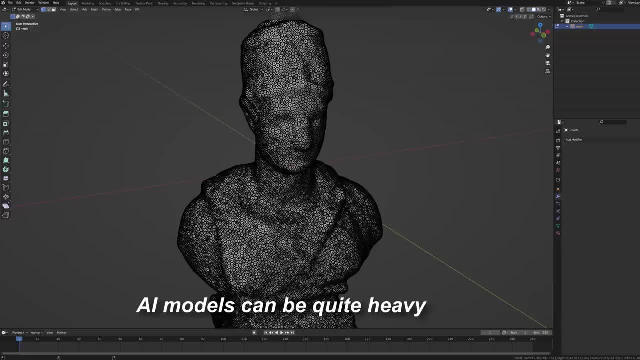 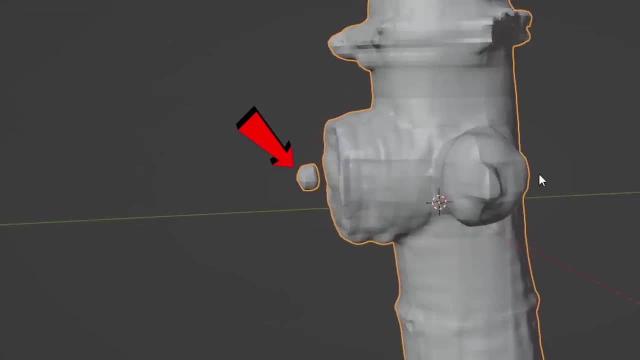 Find the previously saved model and click Import. If your model is highly detailed, it may take a few seconds to process it. Some models will have floating parts which we must get rid of And to do that, select your model. Select your model and click Tab. 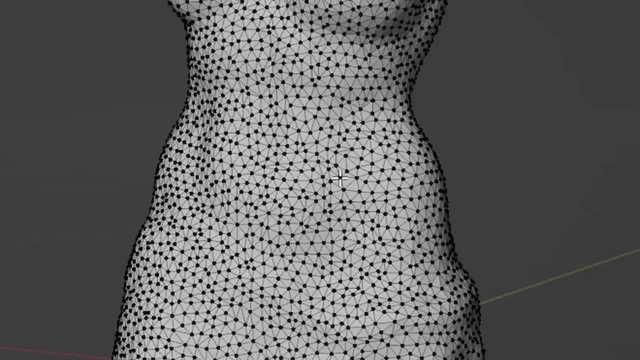 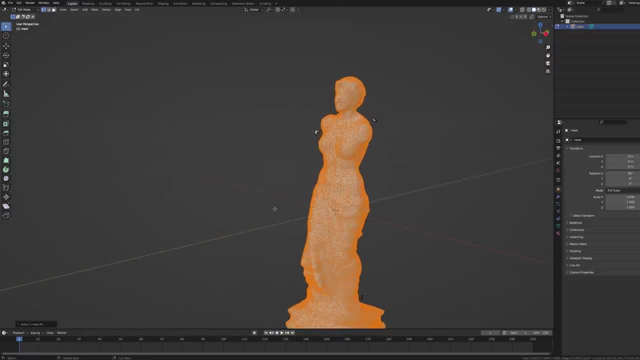 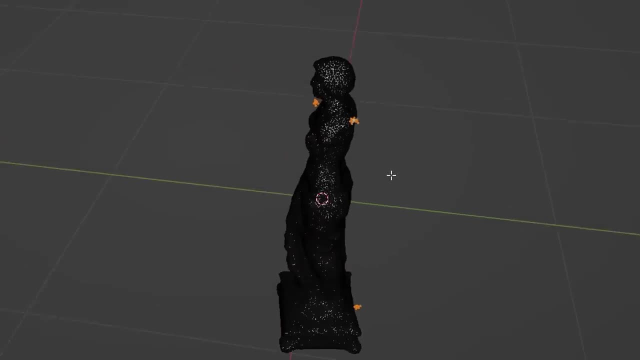 Now press 1 on your keyboard to see the vertices and select anyone that belongs to your model. Now click Ctrl L, which will highlight everything connected within this one object. Ctrl I will reverse the selection to every other object, In other words, all the garbage. 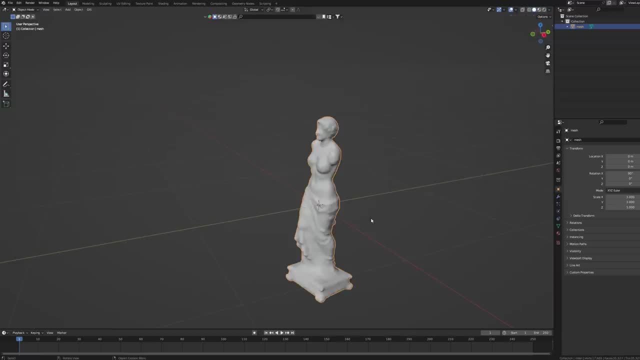 Now press Delete and all the floating artifacts will disappear. Click Tab again To close the Edit mode. Now let's move out our model to make it look better. Select your model, find the little wrench on the right and in the Modifiers menu find. 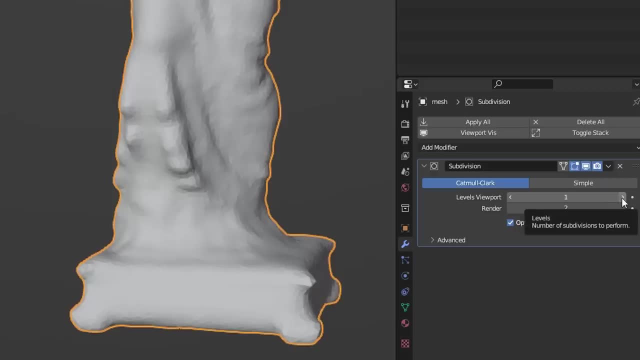 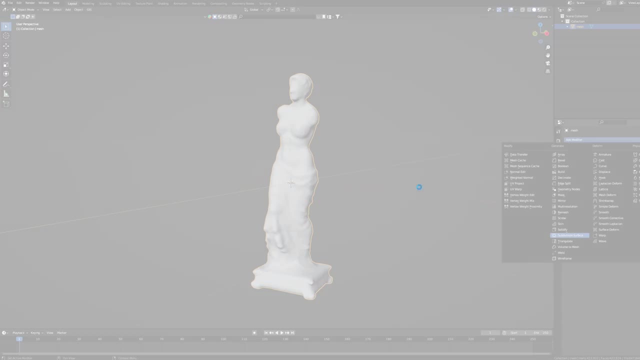 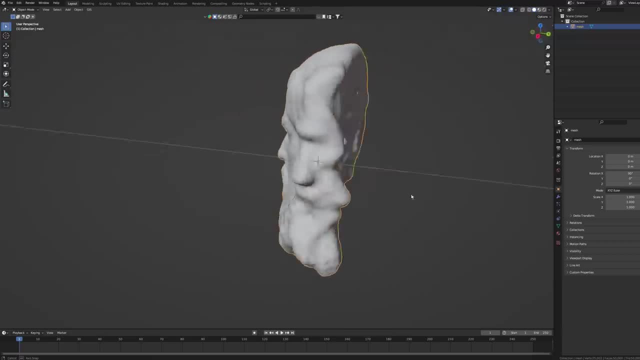 Now, let's choose a side. we want to work as a base. Now, let's choose a side. we want to work as a base. As you can see, the AI-generated models have quite an organic shape. even the flat surfaces are not exactly flat, which can be annoying. 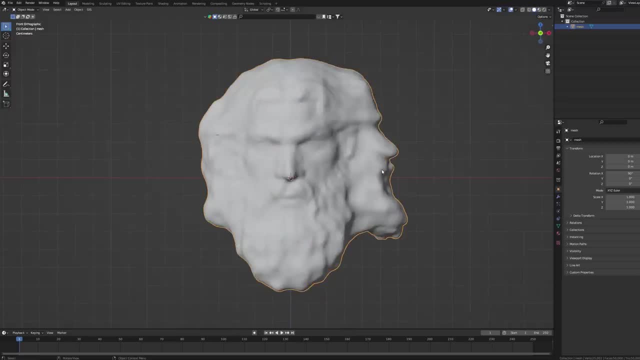 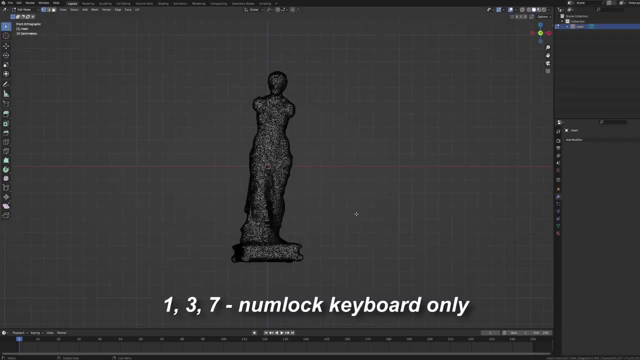 After all, you don't want your 3D print to waggle on an uneven surface. To fix it, select your model and click Tab to go into Edit mode. By pressing 1,, 3 or 7 on your NumLock keyboard, you can switch to Front Side or Top view. 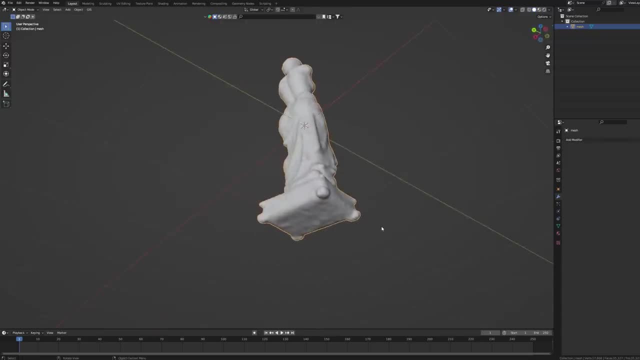 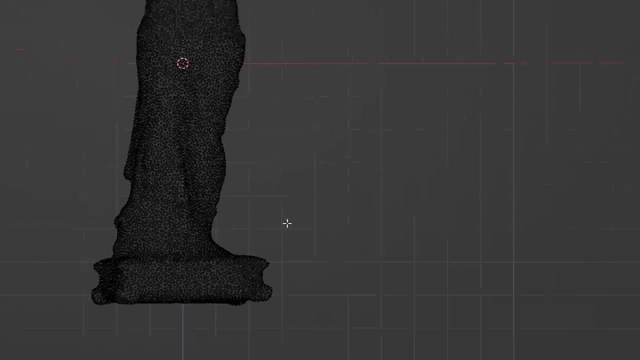 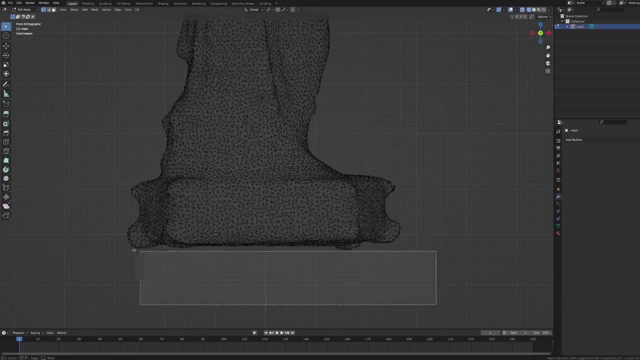 Let's say I want this side to be completely flat. Let's say I want this side to be completely flat. I will now press the Z button and, while holding it, select the wireframe mode with my cursor. Make sure you are working on vertices and then select a bunch of them near the bottom. 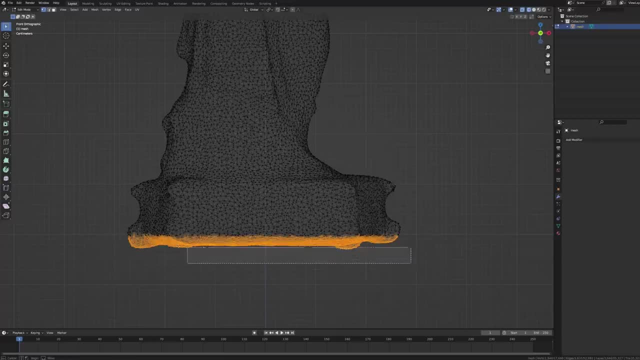 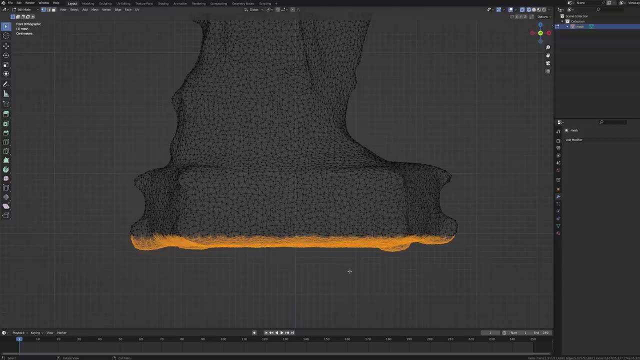 Make sure to make it a straight line and to grab just enough vertices to cover the whole bottom. Now we will scale it in just one direction. For me it will be the Z axis, So I press S, then Z and follow with 0.. 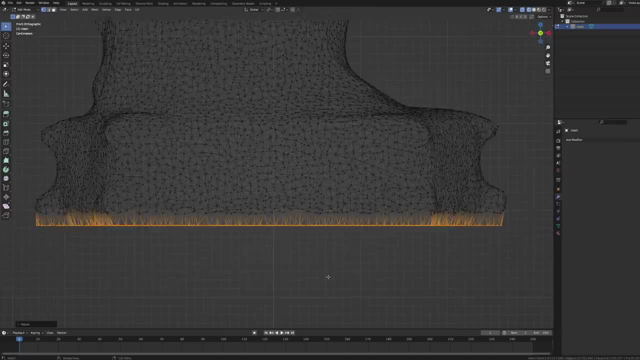 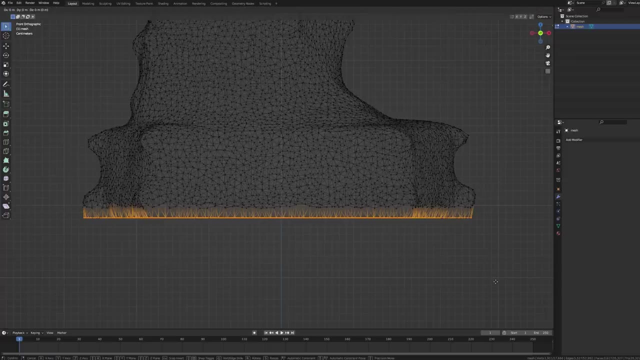 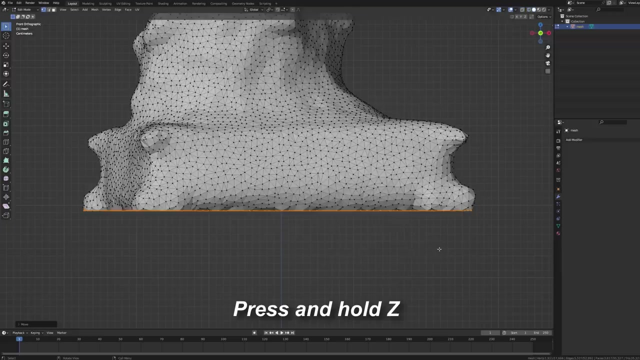 This combination literally means scale only in Z axis, scale to 0, which is flat. You can also move base of your model up or down with G and X, Y or Z. Hold Z, move cursor to the right and click Tab to exit Edit mode. 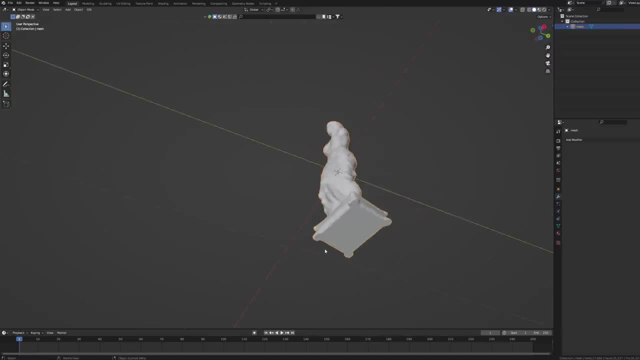 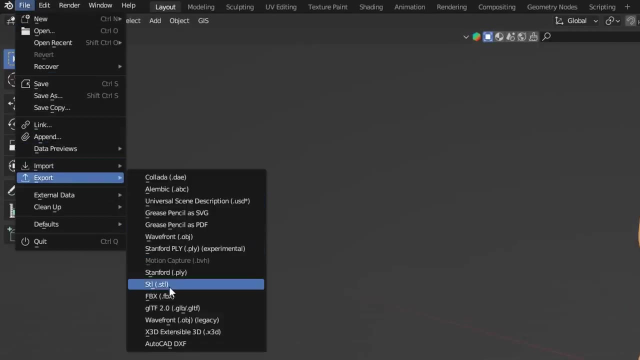 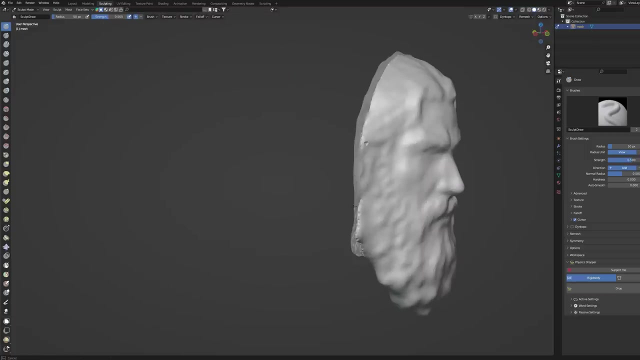 And there you go. Your model is ready for printing, So let's save it. Select the model, go to File Export, STL, and save it wherever you like. If you're feeling creative, you can also modify the models to your own liking. 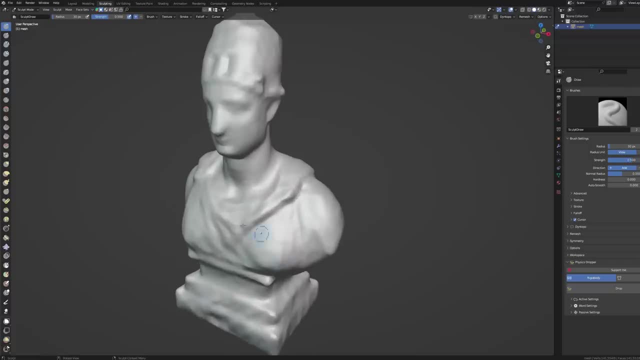 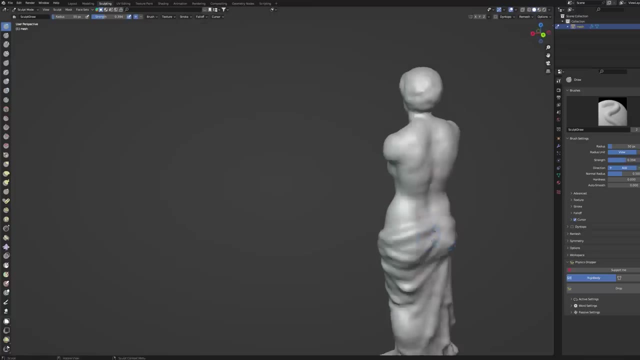 I usually play with the sculpt mode and other features to make the details crispier, but this is a material for another video. If you wish to see a tutorial and more advanced tips on how to enhance your model before 3D printing, please say so in the comments. 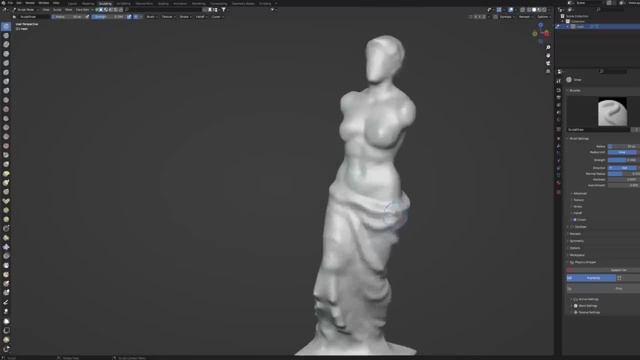 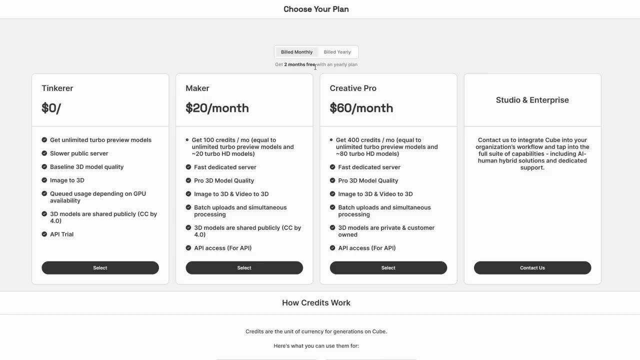 It is important for me to know what would you like to see next. You can have a lot of fun experimenting with CSM AI And, if you choose to, you can access other features like video to 3D model service or faster processing of your models. 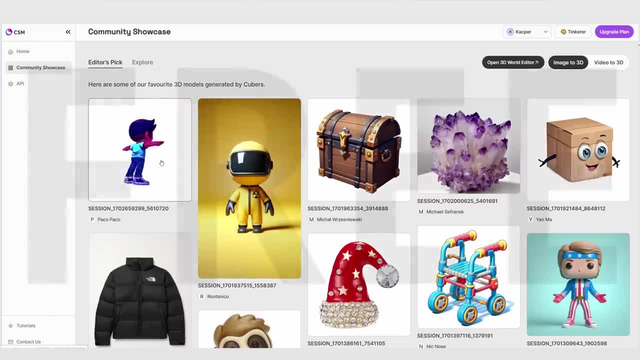 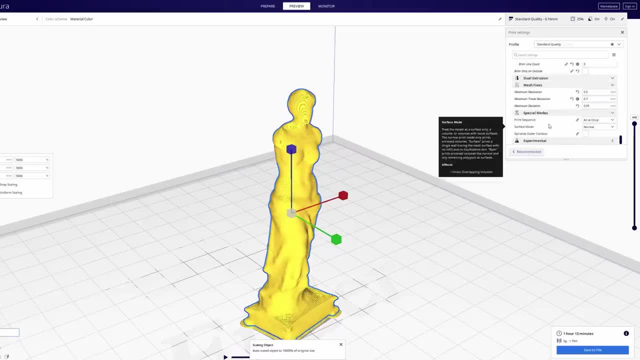